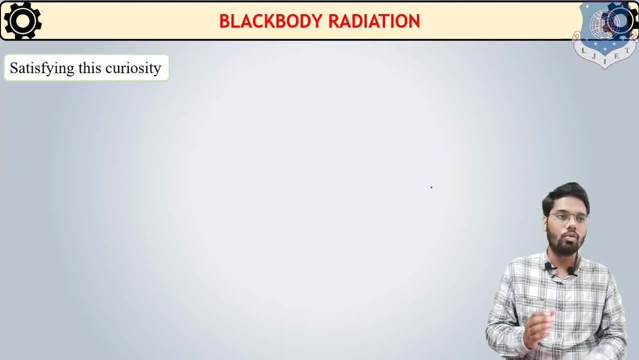 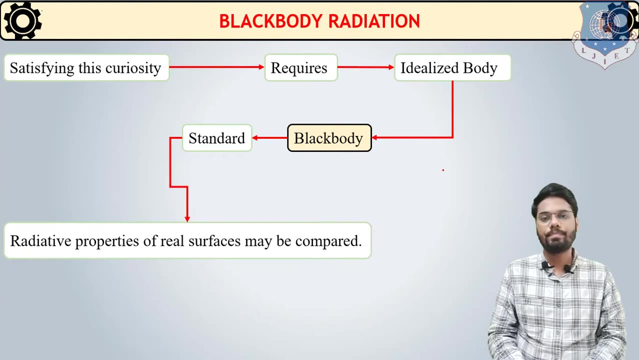 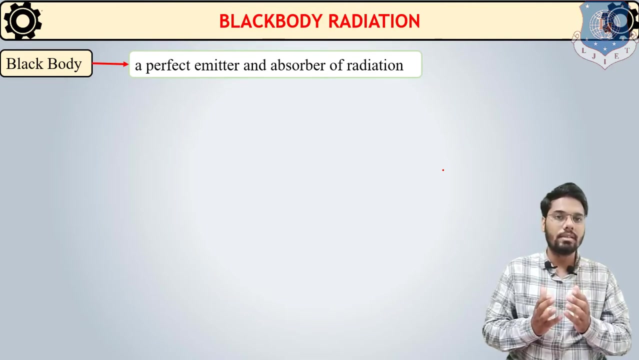 reference to satisfy our curiosity. and that reference point, to which actual body emission can be compared, is known as the black body. This is idealized body In the black body. it is our standard to which another radiative properties of the real surface may be compared. So a black body. it is a perfect emitter and absorber of radiation. It means a black. 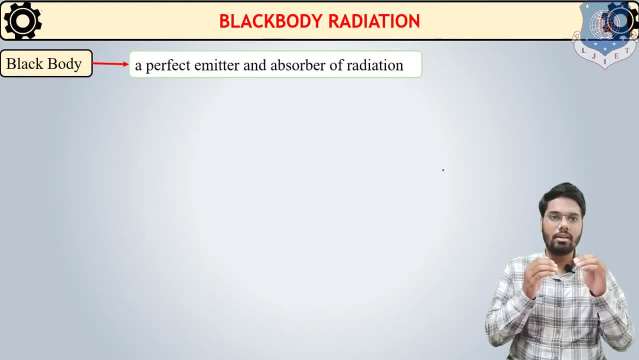 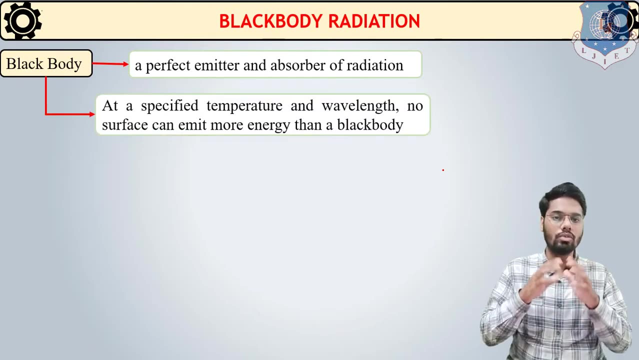 body will absorb all the electromagnetic wave which incident on that body. It will emit electromagnetic wave of full range of spectrum of electromagnetic wave in all the directions At a specified temperature and wavelength. no surface can emit more energy than a black body. Suppose we have two bodies: one is a black body and one is another real body. The temperature of 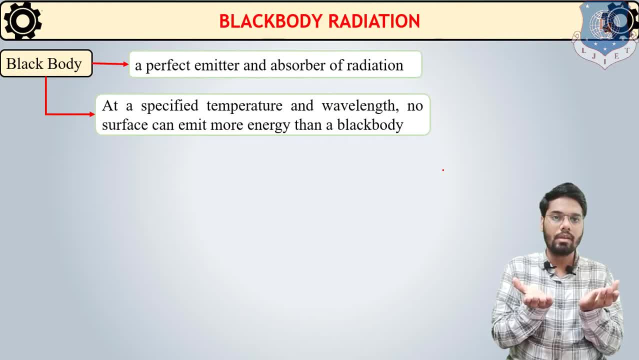 both bodies are same, suppose 60 degree. So at 60 degree the maximum amount of energy, of electromagnetic wave emit by the black body as compared to the real body. So at a specified temperature and wavelength no surface can emit more energy than a black body. Black body absorb. 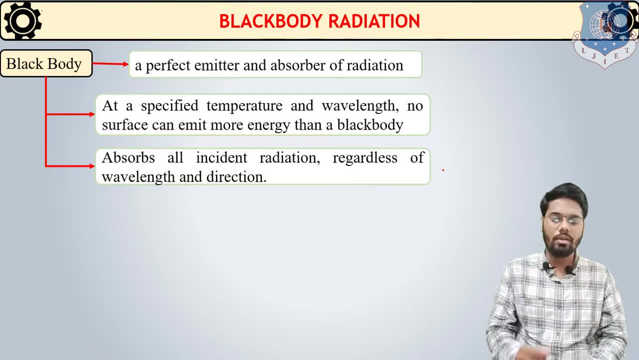 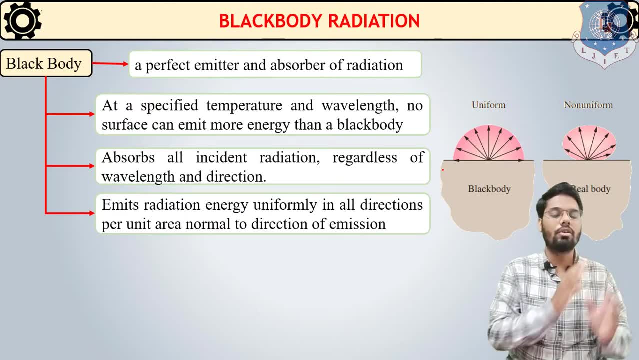 all the incident radiation, regardless of wavelength and direction, as we have just discussed. It emits radiation energy uniformly in all the direction per unit area normal to the direction of the emission. As we can see from this figure, a black body is going to emit electromagnetic wave. 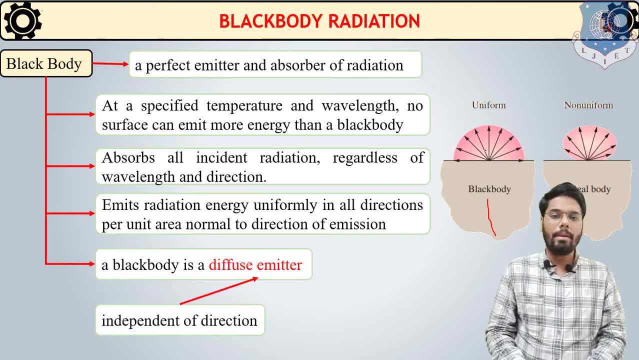 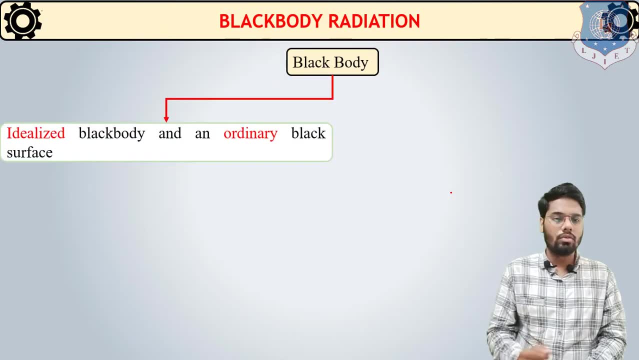 in all direction in uniform way. So a black body is a diffuser emitter. Diffuser emitter means it is independent of the direction. It emits same intensity of electromagnetic wave in all the directions. Now, so in some black body is idealized body. but we have to differentiate. idealized 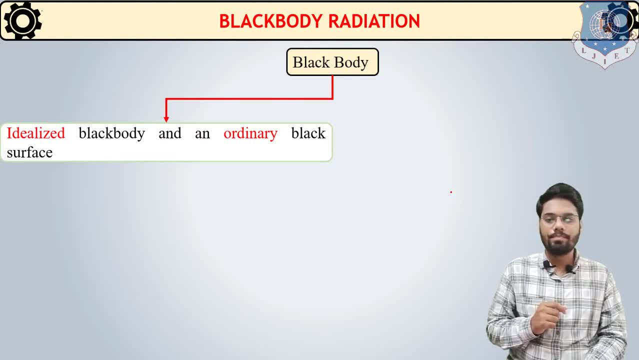 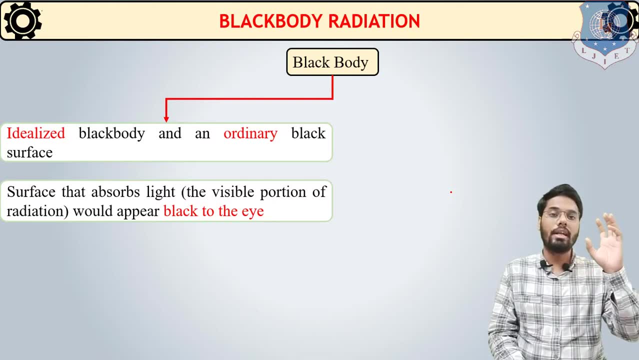 black body with ordinary black surface Because a surface that absorb all the light visible range of light which is in a electromagnetic spectrum. the visible range is 0.4 to 0.76 micron. So 0.4 to 0.76 micron of electromagnetic wave is absorbed by some body, it will appear black to our eye. 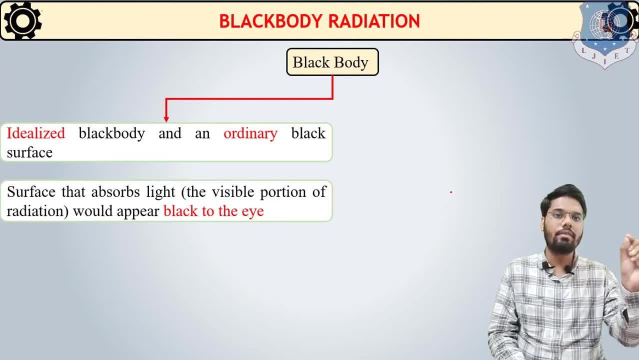 because our eye has a limit of 0.4 to 0.76 micron of wavelength of electromagnetic wave. So the object which absorb all the electromagnetic wave of that particular narrow bandwidth range of 0.4 to 0.76 will appear black to our eye. But that doesn't mean that object is a black body. Suppose 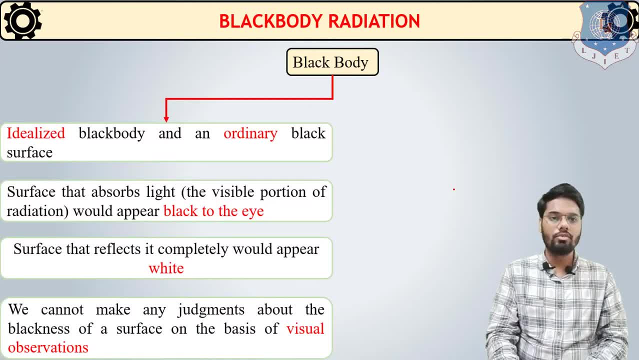 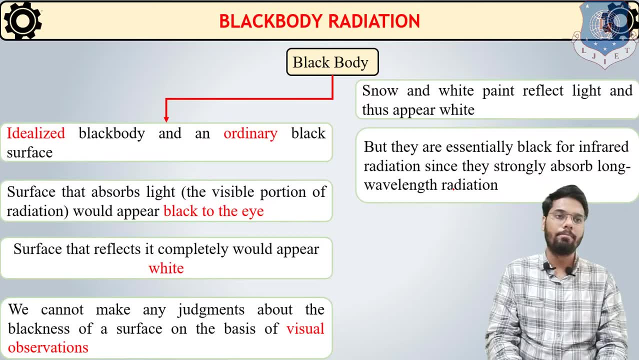 we cannot make this statement about the blackness of the surface on the basis of visual observation, because snow and white paint reflect light and thus appears white, because it will reflect all the visible range of wavelength of electromagnetic wave from 0.4 to 0.76 micron, But same snow and white paint absorbs all three. 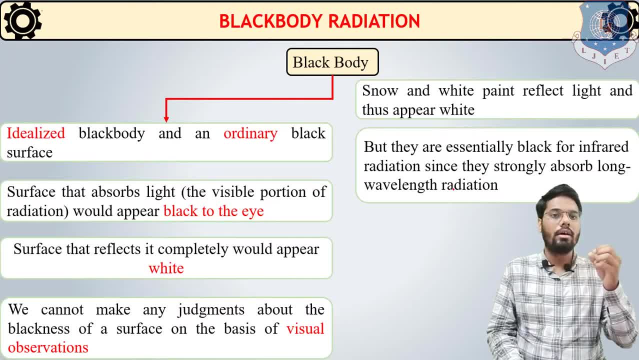 infrared radiation, all three infrared range of electromagnetic wave. So for the infrared range of spectrum that snow and white paint is black, but for the visual range it will appear white for the our eye. so we cannot make judgment about the blackness of the surface on the basis of our 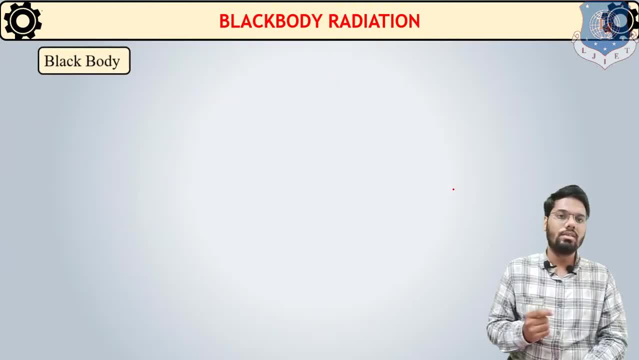 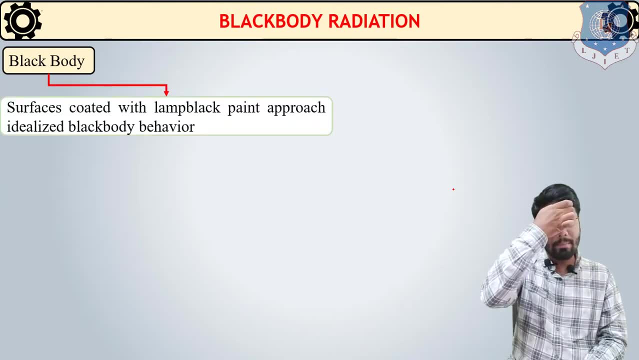 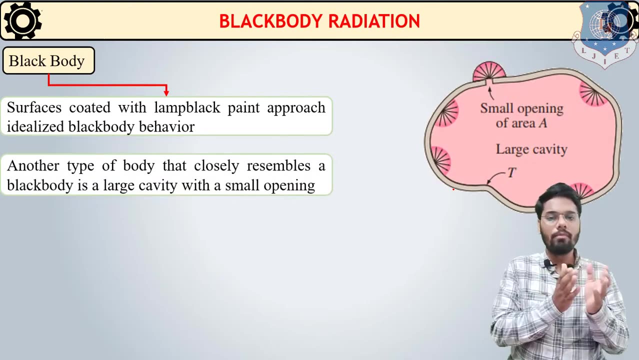 visual observation. so the question is: what is the real body that resemble closeness to the black body? the surface coated with the lamp? black paint approaches idealized black behavior, black body behavior. another type of black body that closely resemble a black body is a large cavity with a 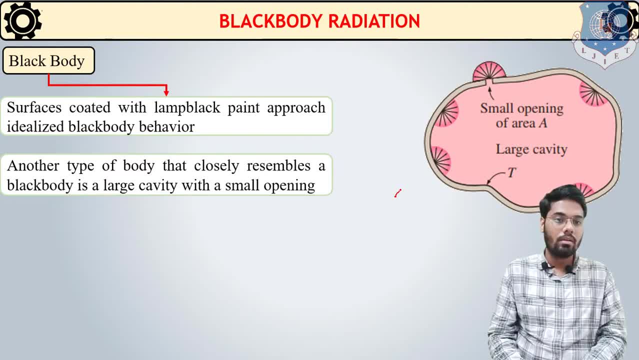 small opening, as we can see here from this figure. a electromagnetic wave which comes in from this little opening will reflect number of times before escaping. so whenever it reflect number of times, a little portion of that electromagnetic will absorb. so before escaping from this opening it lost almost every energy, every packets of photons within this cavity. so this cavity will 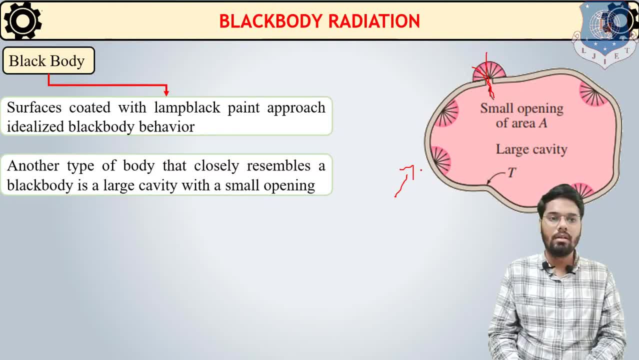 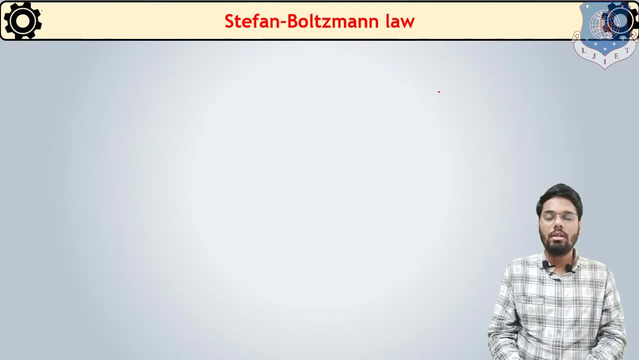 closely behave like a black body if we are iso, if the temper, if this body is isothermal at temperature t. now there are different laws related to the radiation. first one is the stiffen voidsman law we have just discussed. let's sum up what we have learned. 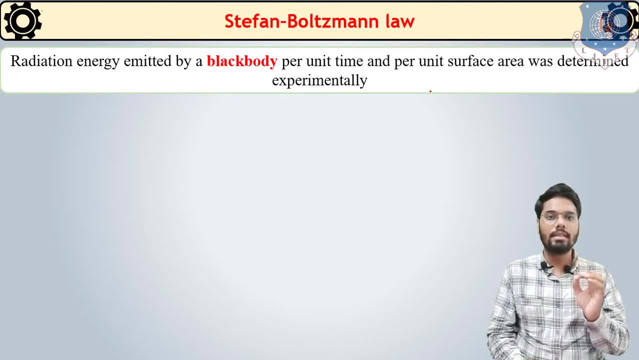 to this point, everybody whose temperature is about absolute zero emits electromagnetic wave. that electromagnetic wave contains packets of photon, or we can say that the energy, so everybody whose temperature is about absolute zero emits electromagnetic wave of different wavelength, of different energy. because we know from the relation that the 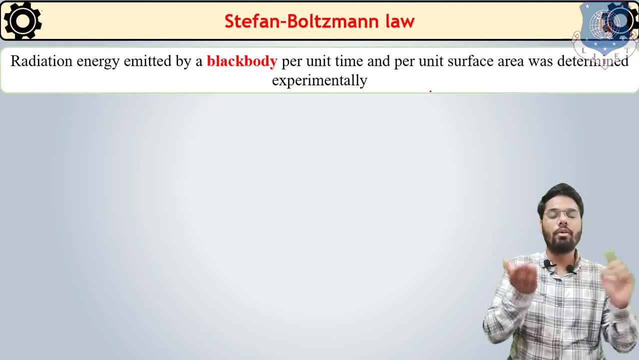 smaller the wavelength, higher the energy contains by the electromagnetic wave. so the question is, whose electromagnetic wave consider larger energy? so wavelength of the electromagnetic wave depends on the different parameter, like temperature of the surface, surface conditions as well as the material of the surface at same temperature if there are two bodies. 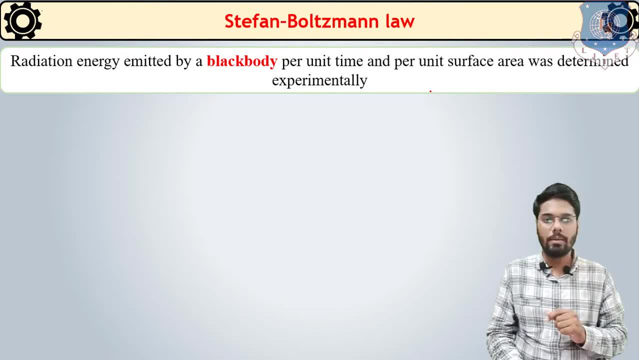 one body emits more electromagnetic wave as compared to the another body. so, for the comparison, one idealized condition, one idealized body that is known as the black body. a black body emit is a perfect emitter as well as perfect absorber. it means it will absorb all the electromagnetic wave. 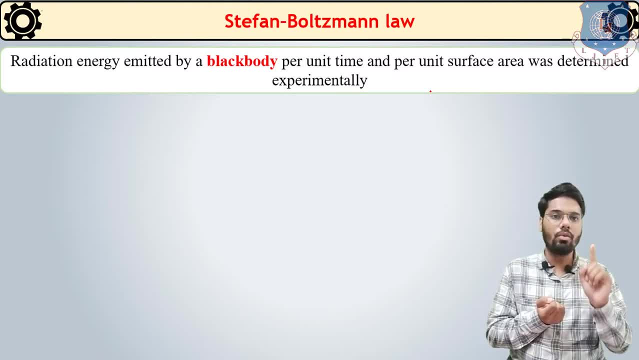 which incident on it, as well as at a particular temperature. black body emits maximum amount of electromagnetic wave as compared to all other bodies, so it is a perfect emitter. now we required one equation from which we can calculate the emissive power. emissive power means electromagnetic wave emitted by a black uh, by a particular body, per unit time, per unit area. 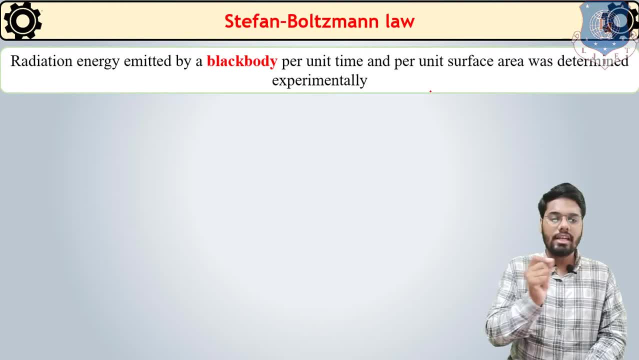 so experimentally. it is uh radiation energy emitted by black body per unit time and per unit surface area was determined by joseph stephen in 1879, which is given by eb. it is emissive power of the black body is directly proportional to 10. 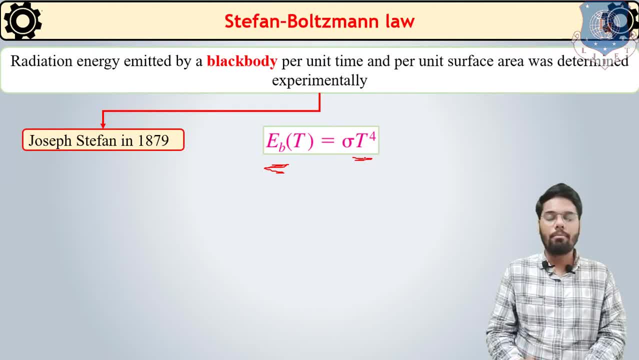 temperature is to 4. temperature t is a temperature of the black body surface. so if we remove proportionality limit from this equation, we have to put one constant, which is sigma, which is known as the stephen boltzmann constant, whose value is 5.67, into 10 raise to minus 8 watt per meter square. 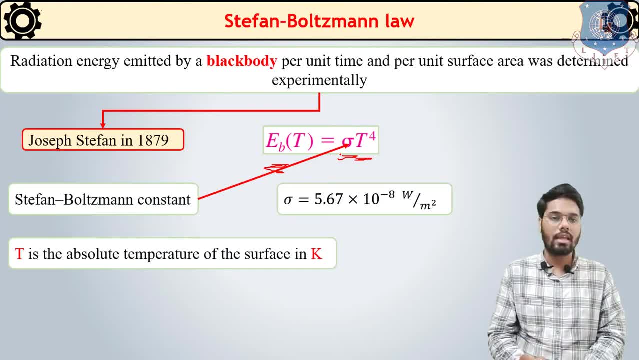 here t is the absolute temperature of the surface of the black body in a kelvin and eb is a black body emissive power. so from this equation, at particular temperature, we can easily find out emissive power of the black body and the black body. emissive power of the black body is equal to. 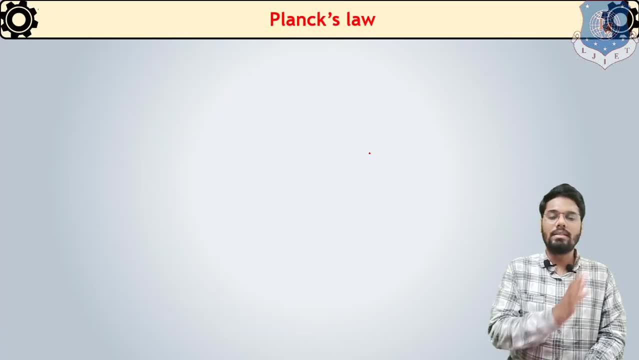 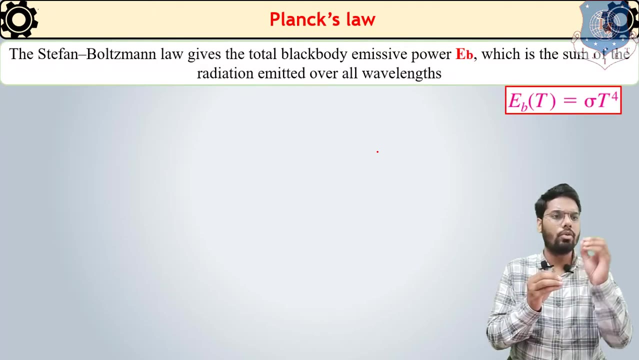 the black body. now there is another law, which is plant snow, because at particular temperature a body emits a wide range of wavelength, of electromagnetic wave, but in some cases we are only interested in a particular wavelength. suppose if a light bulb emits electromagnetic wave at particular temperature, but we are more interested only in a 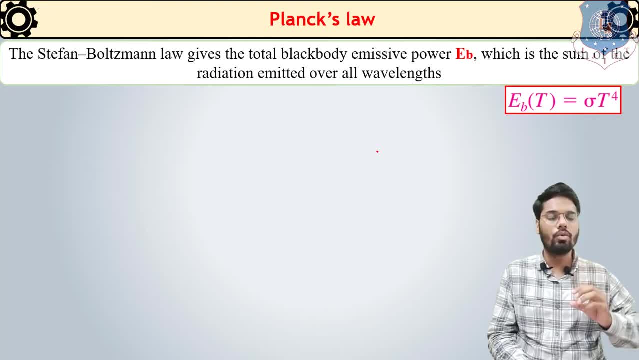 particular visible range for the light bulb. we just want to know how much amount of electromagnetic wave is emitted by the light bulb, whose wavelength is between 0.4 to the 0.76 micron, because this is the only range which is visible by the human eye. we are not interested in another other wavelength. 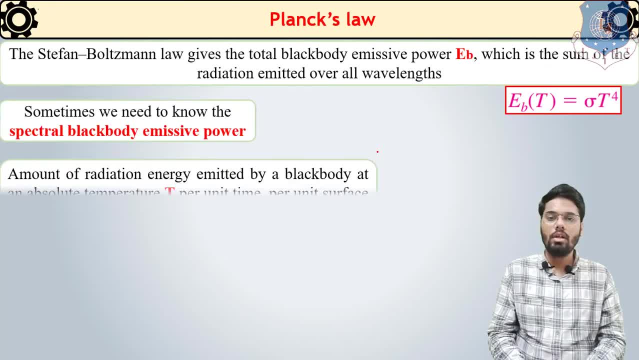 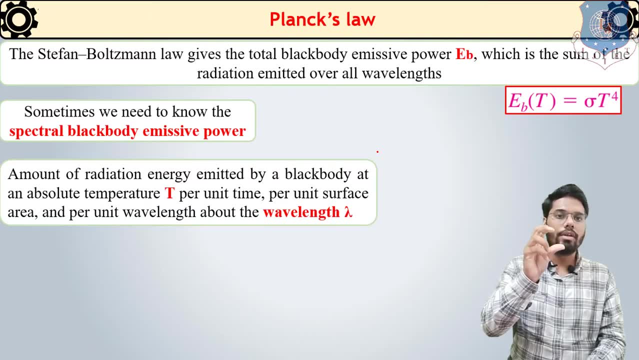 than four, point four to the point seven, six micron, so that emissive power, or that power which is emitted within the 0.4 to points, because of 0.4 to 0.76 micron of wavelength, is known as the spectral black body emissive power. so here as written: amount of radiation energy emitted by 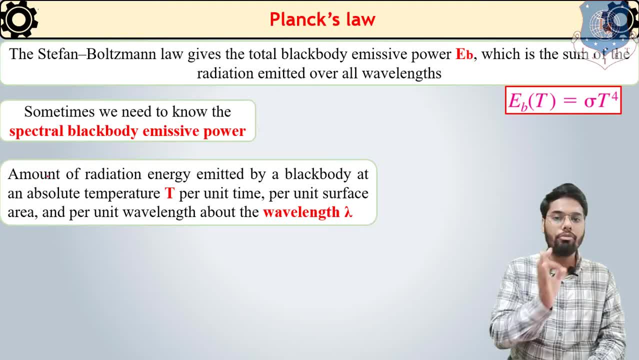 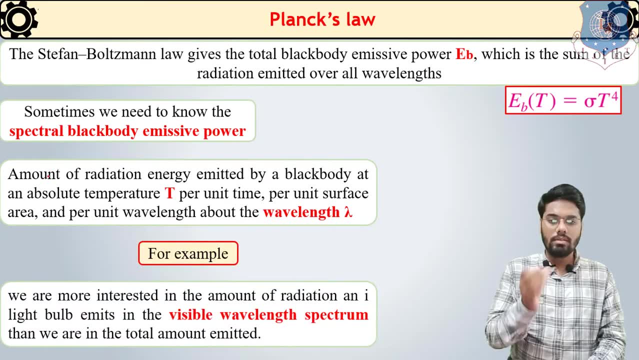 black body at an absolute temperature, t per unit time, per unit surface area and per unit wavelength. about the wavelength lambda, for example, we have just discussed. we are more interested in the amount of radiation and light bulb emits in the visible wavelength spectrum of the black body. so 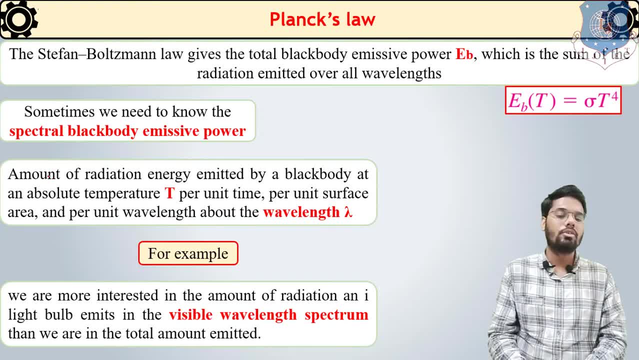 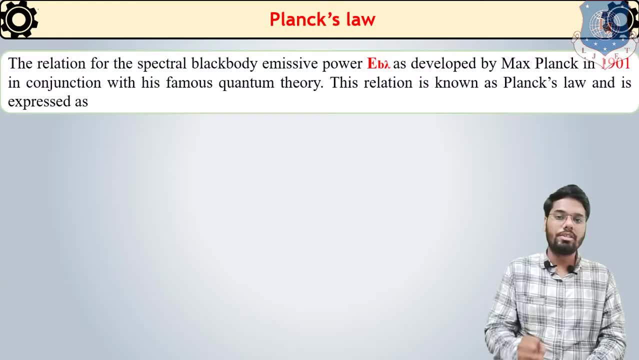 we are more interested in the amount of radiation and light bulb emits in the visible wavelength spectrum than we are in the total amount of emitted, total amount of electromagnetic wave emitted. so the that equation, the relation for the spectral body, emissive power, eb lambda. eb lambda means: 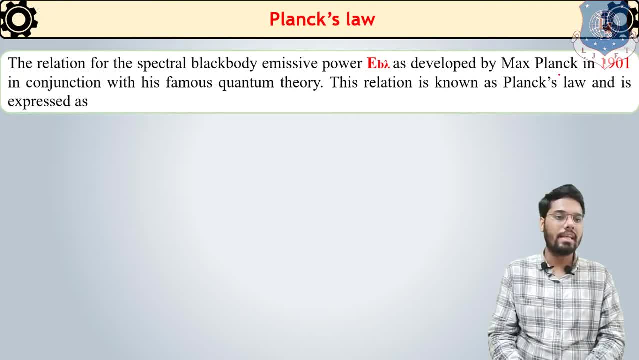 emissive power of particular wavelength lambda is developed by max planck in 1901 in conjunction with the famous quantum theory. this relation is known as the planck's node. it is expressed as eb- lambda at particular temperature. this lambda comma t represents wavelength at particular. this temperature is equal to c1 divided by lambda raise. 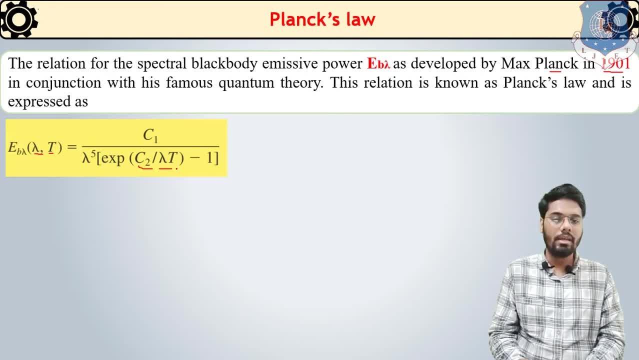 to 5 in bracket exponential of c2 divided by lambda t minus 1.. here c1 and c2 is the constant whose values are as per this, c1 is equal to 3.742 into 10. raise to 8 watt. c2 is equal to 1.439 into. 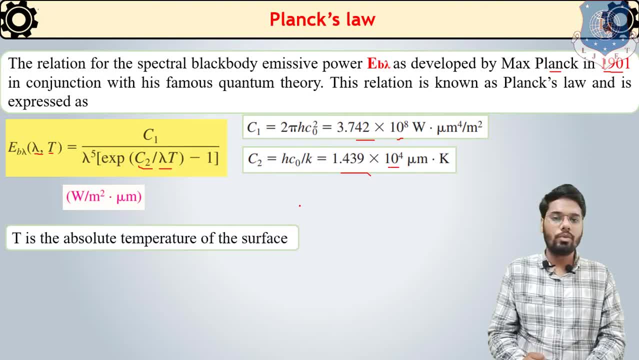 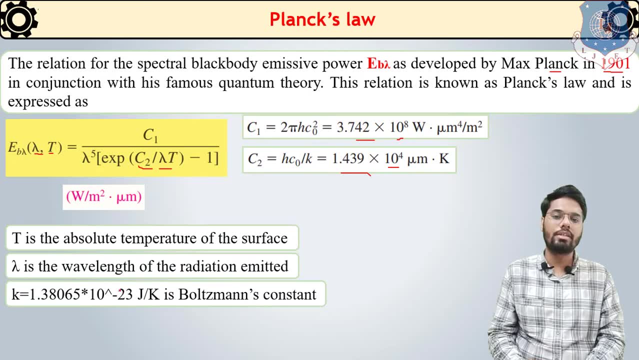 10. raise to 4 micron. here, in this equation, t is the absolute temperature of the surface, lambda is the wavelength of the radiation emitted and k is 1.3 into 10. raise to minus 23, which is known as the boltzmann constant. this relation is valid for a surface in a vacuum or gas. now another law which: 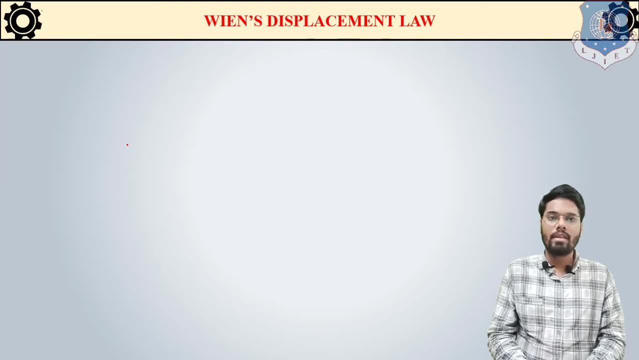 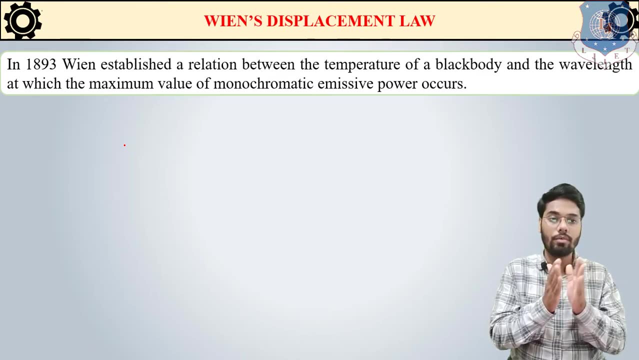 is related to radiation is vane's displacement law. it suggests that in 1893 vane displacement established a relation between the temperature of a black body and the wavelength at which maximum monochromatic emissive power occurs. according to vane's law, everybody at a particular temperature 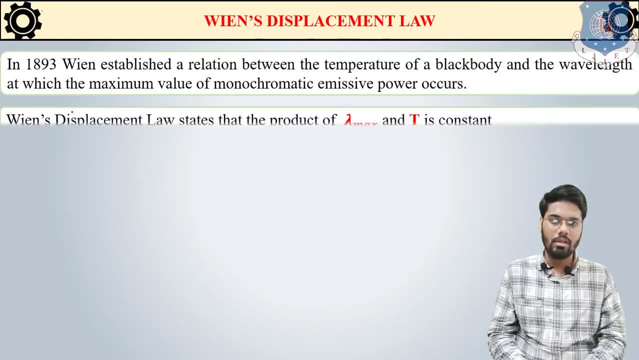 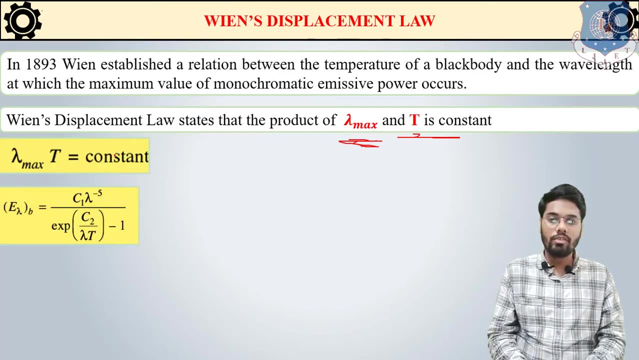 have a maximum wavelength for the emission. so it states that the product of lambda maximum- it means maximum wavelength at particular temperature, t. so product of this lambda max into t is always constant. we can find out value of this lambda max into t by differentiating planck's equation. so here: 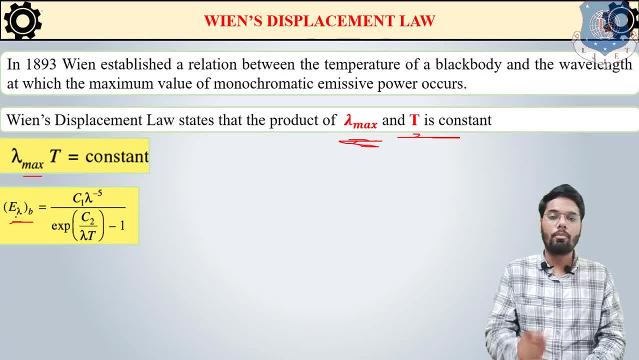 we have written equation which is given by planck for the monochromatic emissive power. so to find out value of this lambda max into t, we have to differentiate this equation with respect to wavelength. it means by the lambda, so d, by d lambda of this equation. 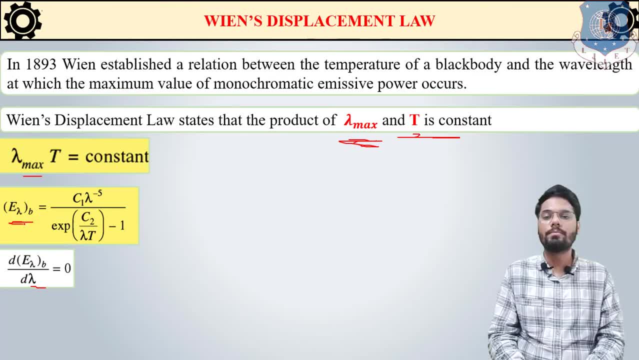 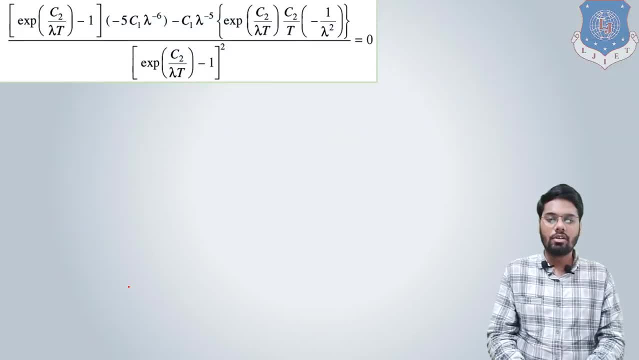 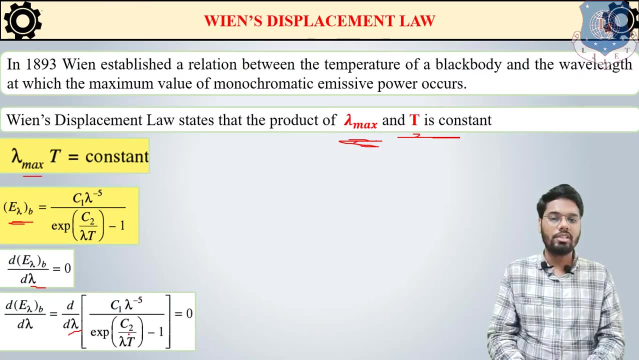 emissive power, of monochromatic emissive power at particular wavelength. so let's differentiate this equation with respect to lambda. so we will get, by differentiation of this equation: uh, in a new numerator we have c1, lambda raise to minus 5, in denominator we have exponential of c2. 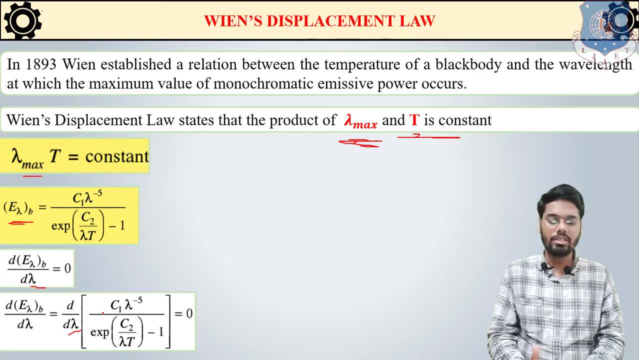 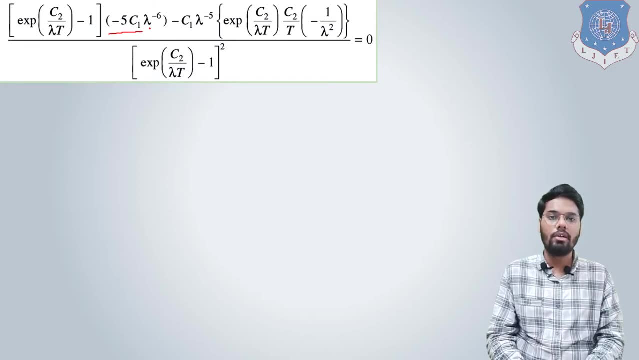 by lambda t minus 1.. So differentiation of this equation would be: first, we will put this denominator as it is and differentiation of this numerator it will c1 into lambda raise to minus 5,. it will give minus 5 into c1 to lambda raise to minus 6,. denominator as it. 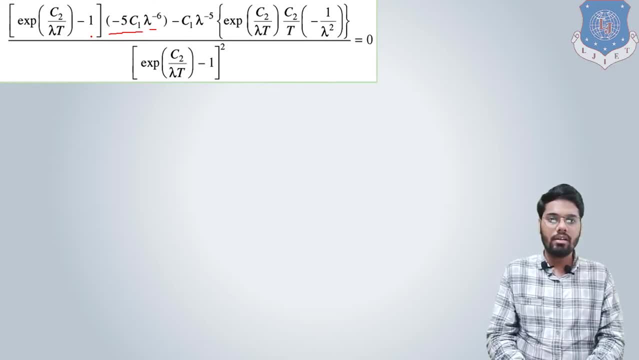 is minus differentiation of denominator, putting numerator as it is c1 lambda raise to minus 5, as it is differentiation of this exponential c2 by lambda t minus 1.. So e raise to something will remain as e raise to something as it is, differentiation of c2 by lambda t will. 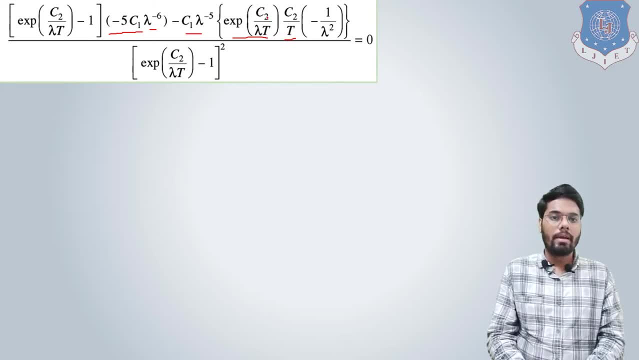 become c2 by t. c2 by t constant 1 minus lambda becomes minus 1 upon lambda square and in upon square of the denominator which is exponential of c2 by lambda. t minus 1 square Equal to 0.. Now if we cross, multiply this exponential term with 0, it will become 0.. 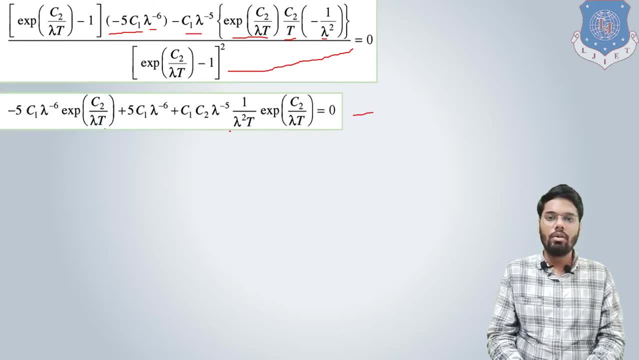 Simplifying this equation. we will get this equation Now here. we can see that here this is a c minus 5. c1 lambda raise to minus 6 minus 5. c1 lambda raise to minus 6, and here c1 lambda raise to minus 5 and 1 upon lambda from this equation gives us a lambda raise. 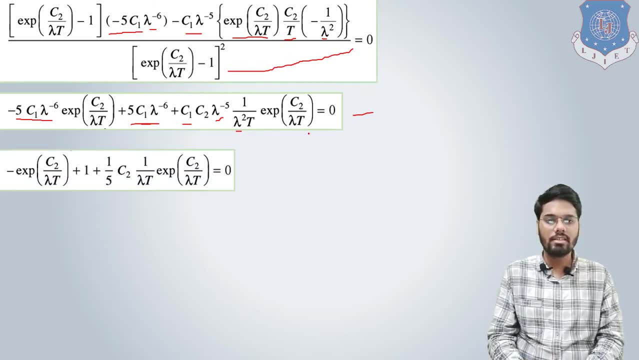 to again minus 1.. So it becomes lambda raise to minus 6.. So, simplifying this equation, we will get minus exponential of C2 by lambda t plus 1 plus 1 upon 5 C2, 1 upon lambda t. exponential of C2 by: 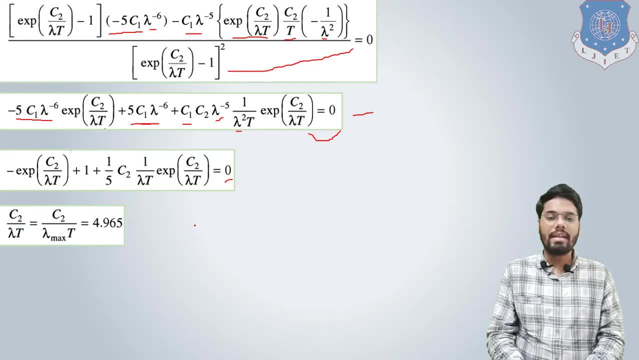 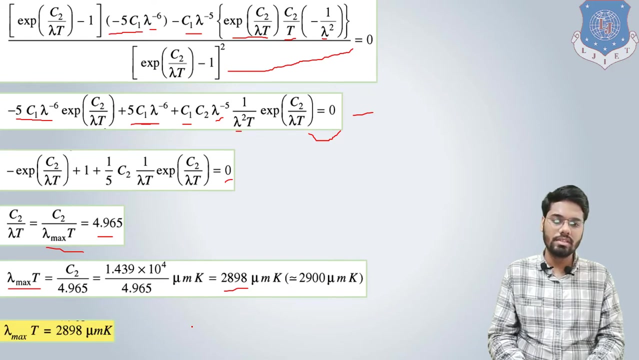 lambda t is equal to 0.. By trial and error method solving this equation, we will get C2. by lambda max, t is equal to 4.965.. Now putting the value of C2 in this equation, we will get the relation lambda max into t is equal to 2898 micron Kelvin. So this is the final equation, final value. 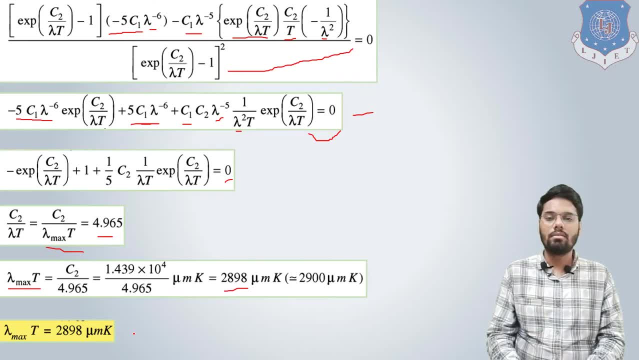 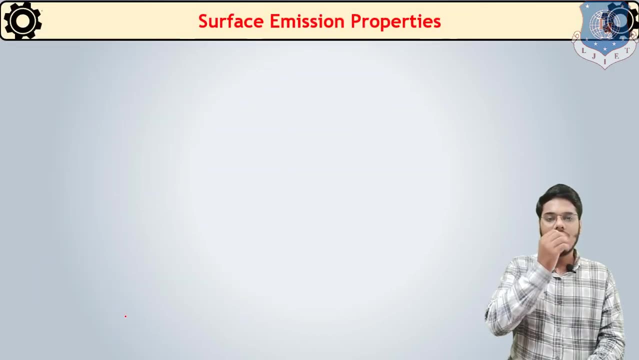 for the Wien's displacement law, which is, which is generated by, which is calculated by the differentiation of Planck's equation, which is: lambda max into t is equal to 2898 micron into Kelvin. Now let us discuss some surface emission properties that are used in the equation. So let us first discuss the surface emission properties. 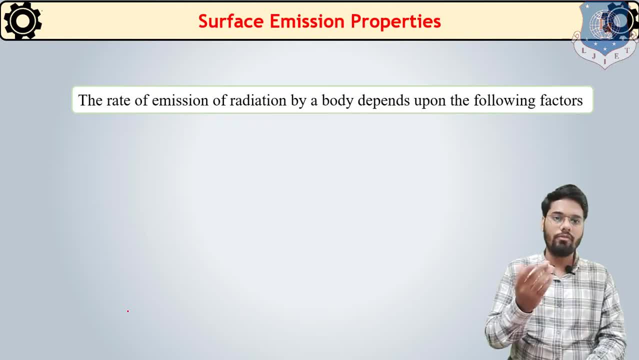 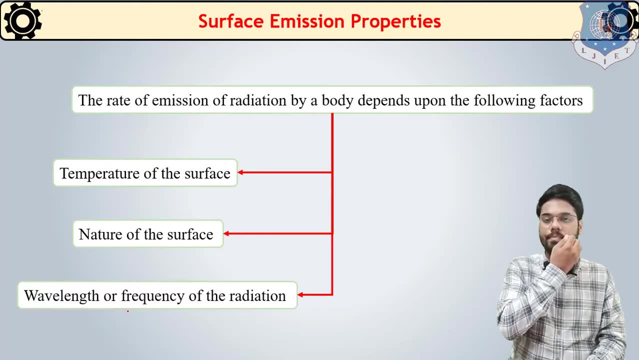 Let us first discuss the surface emission properties that are used in the equation. The rate of emission of radiation by black body depends upon the following factor, as we have just discussed: temperature of the surface, nature of the surface and the wavelength of frequency of the radiation. So parameter which deals with the surface emission properties first, is a total. 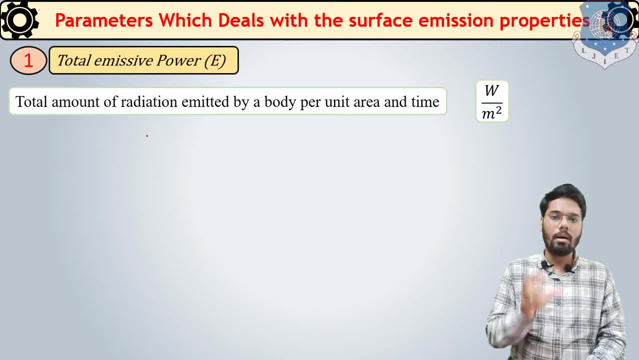 emissive power. Total emissive power means the amount of radiation, total amount of radiation which is emitted by the black body per unit area in time, watt per meter square. It is known as the total emissive power. It represents the whole emissive power of the black body. So the total. 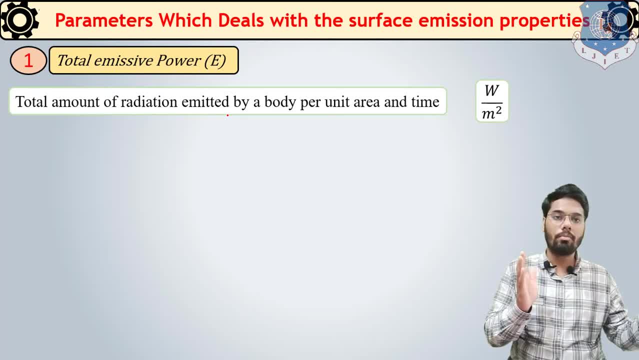 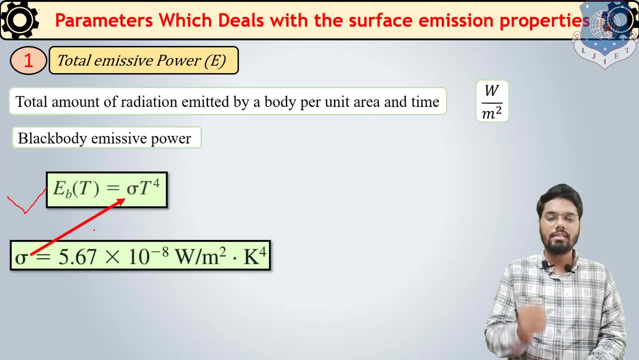 energy emitted is the total emissive power. by all the range of wavelength of electromagnetic wave which is emitted by any body, It is known as the total emissive power. and for the black body emissive power we know the equation which is given by Stefan Boltzmann is: EB is equal to sigma, t is equal to 4.. 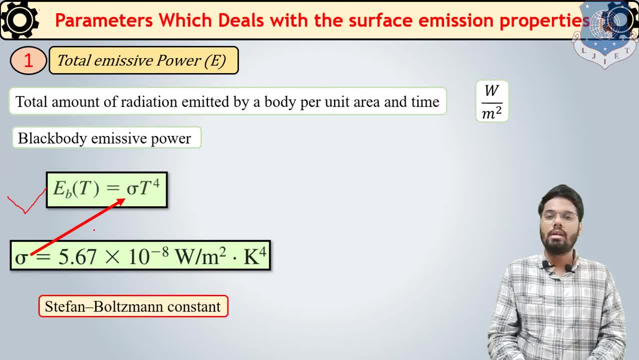 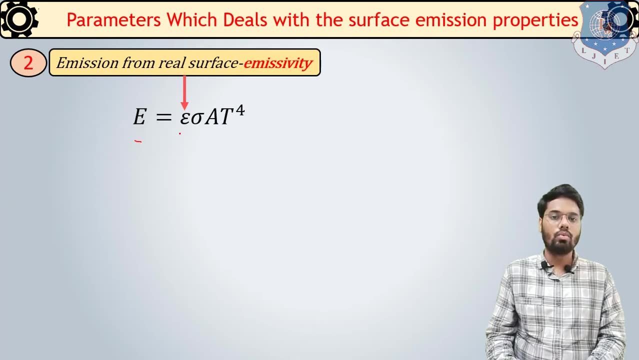 Here, sigma is Stefan Boltzmann constant, whose value is 5.67 into 10 is to minus 8.. Now, second is the for the black body, now for the real surface, the equation will become capital. E is equal to. this is emissivity of a real surface. this epsilon is emissivity of the real surface into Sigma, into 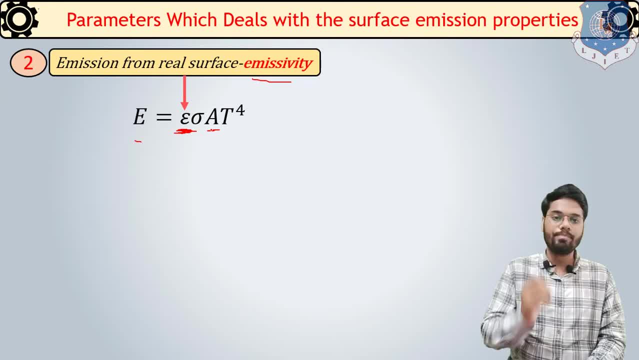 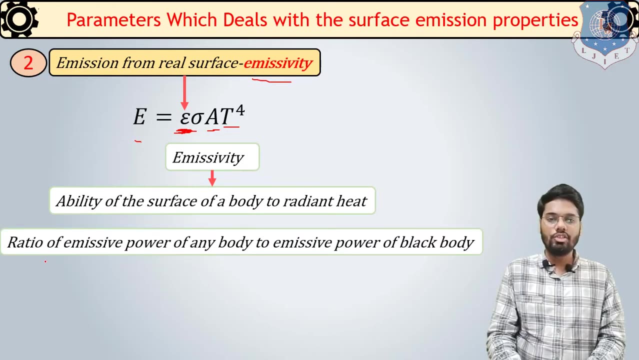 area. this is the area, real area of the body and this is the temperature is to for temperature of the body. here, this is the emissivity, it is the ability of surface of the body to radiate or the to emit the electromagnetic wave or to emit the heat. ratio of emissive power of any body to the 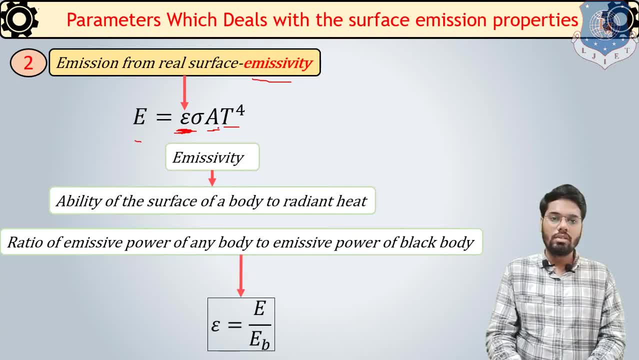 emissive power of the black body, because we know that this Sigma into area, into T, raised to 4, is our black body emissions. so e by e, B is known as the emissivity of any body. it is the ratio of emissive power of any body. 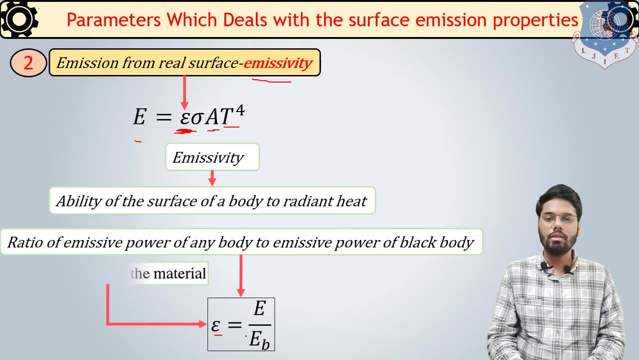 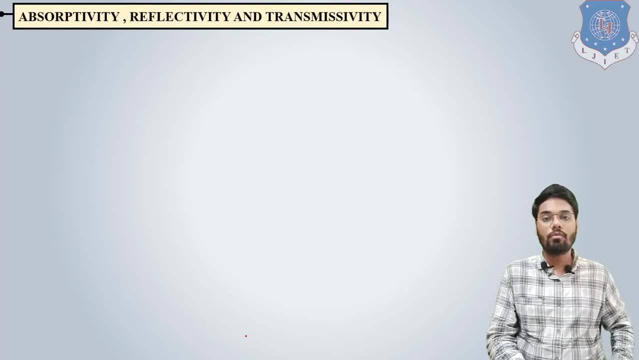 to the emissive power of the black body. it is known as the emissivity of any material. now, as we know that electromagnetic wave is responsible for the radiation mode of heat transfer, so it is wave. so when one electromagnetic wave which is emitted from the body, one and it incident on 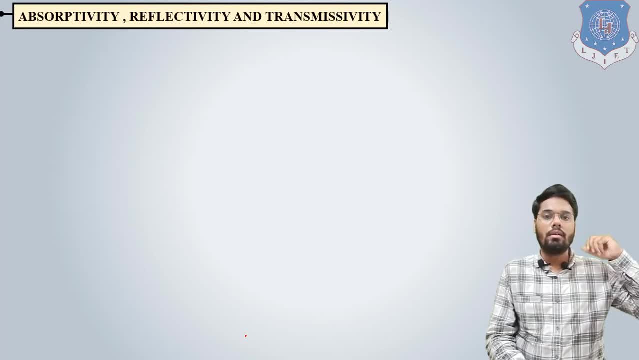 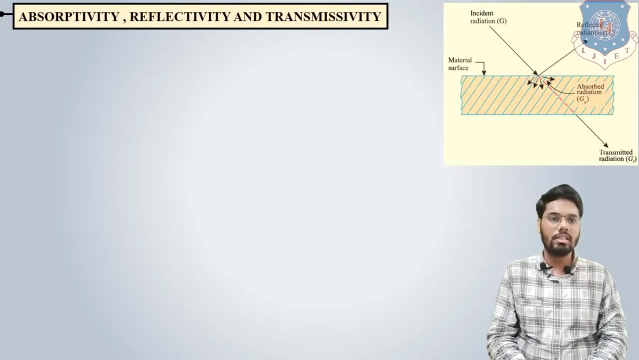 another body, another surface of the body. two: there are some wave properties like absorptivity, reflectivity and transmittivity. so let's discuss that. suppose in this figure we can say that that there is an incident radiation capital G, it will incident in this surface. now there will be three. 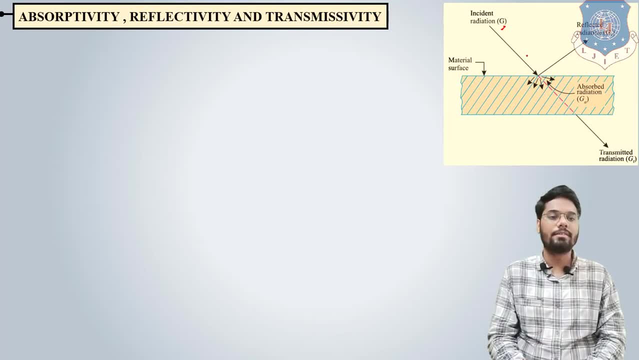 phenomena which will occur. for this rate, incident radiation. for this incident electromagnetic wave. some portion of this wave will reflect, some portion of this wave will transmitted through this body and some portion of this wave may be absorbed by the body. so the total amount of wave which is incident on this body is capital G. now, from this capital G, 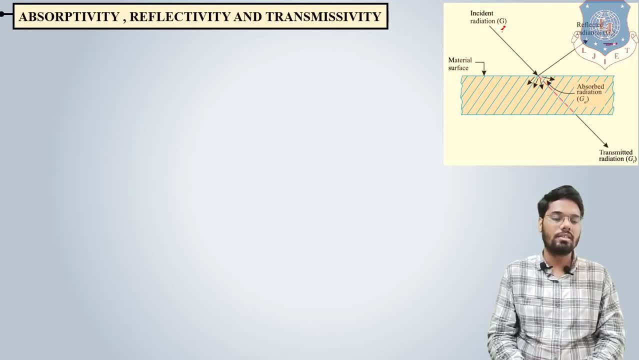 some portion will reflected, which is denoted by G suffix in suffix R. some portion will absorb, so capital G in suffix A, and some portion will transmitted through the surface, through the material, so capital G in suffix small t. total amount of G, which is divided in three parts. 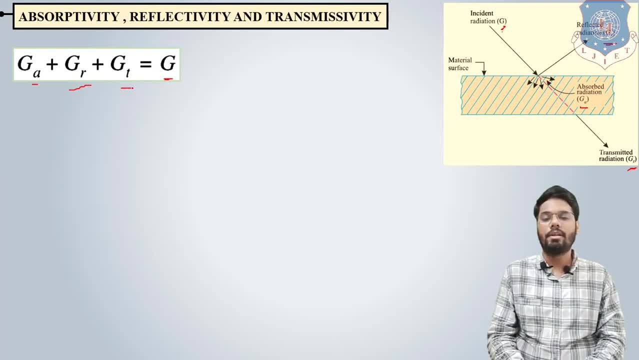 some will absorb, some will reflect and some will transmit. so dividing this equation with capital G in both side, we will get this equation. in this equation, this G A by total G amount of electromagnetic wave is absorbed, divided by total amount of incident, is known as the alpha, which is absorptivity. this G R by G amount of. 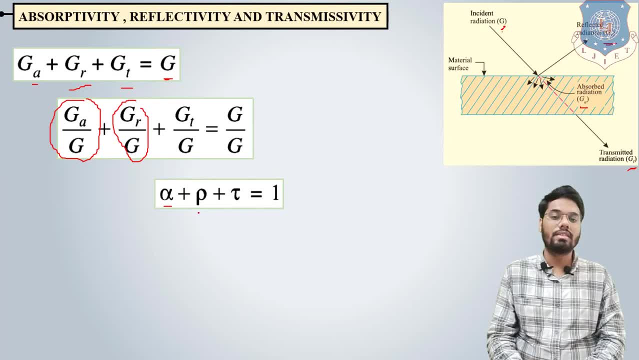 radiation which reflected, divided by total amount of radiation, is known as the rho, which is reflectivity. G, T by G, this is the amount of radiation which is transmitted divided by total, is known as the transmitivity denoted by tau, and this G A by G is equal to 1, so for any body, 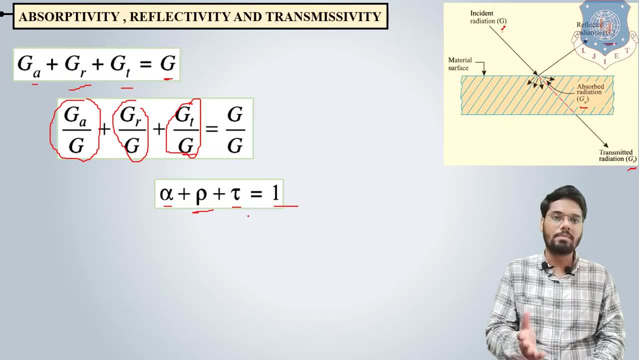 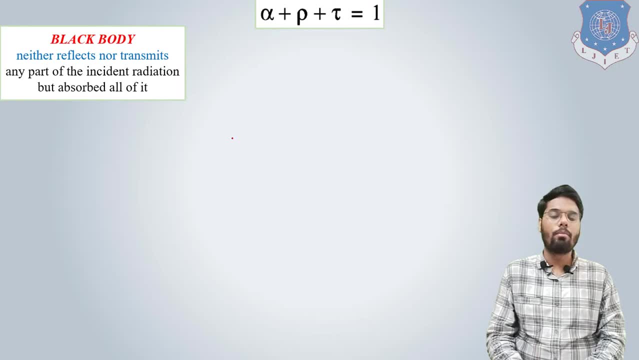 alpha plus rho plus tau, absorptivity plus reflectivity plus transmitivity- is equal to 1. okay, now in this equation for a black body. black body neither reflects nor transmit. it will absorb all the radiation which is incident on it. so for the black body, alpha is equal to one, because it. 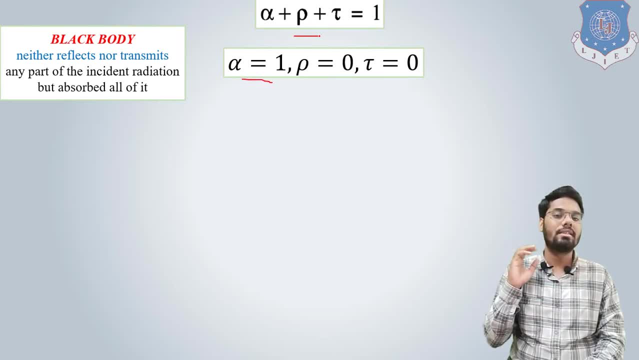 absorb all the radiation. it will not reflect any radiation. it will not transmit any radiation. so for black body, alpha is equal to one, because rho and tau is zero. for opaque body, no incident radiation is transmitted. so for opaque body, tau is equal to zero. so from this equation, alpha plus. 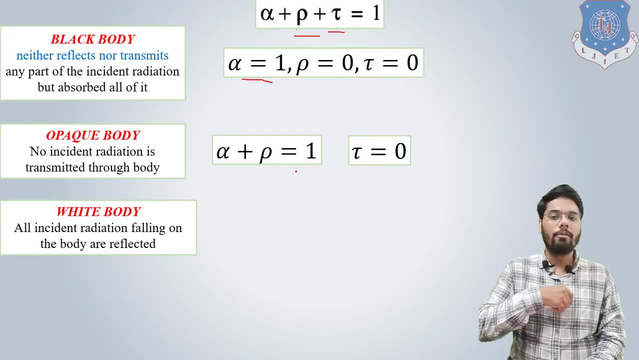 rho is equal to one for a white body. white body will reflect all the radiation falling on the body. so for white body, alpha is equal to zero. there is no absorption, there is no transmittivity, so tau is equal to zero. so for white body, rho is equal to one. reflectivity is equal to one. 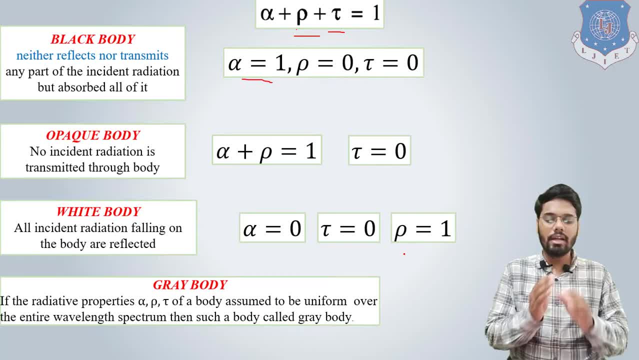 for a gray body. now, if the radiative properties alpha, rho and tau of a body assumed to be uniform over the entire wavelength spectrum, then such body is known as the gray body. again, i repeat it. what is gray body? a body which have radiative properties alpha, rho and tau. 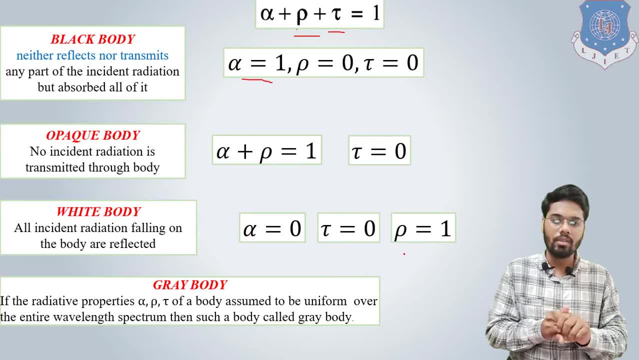 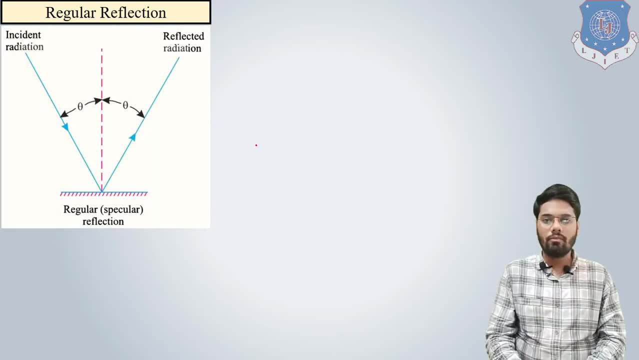 assumed to be uniform over the entire wavelength spectrum, then that body is known as the gray body. now there are two kind of reflections. one is a regular reflection. as we can understand from this figure the angle which is made by the incident radiation with this reference line and the reflector radiation is the same, then it is a known as the regular reflection. 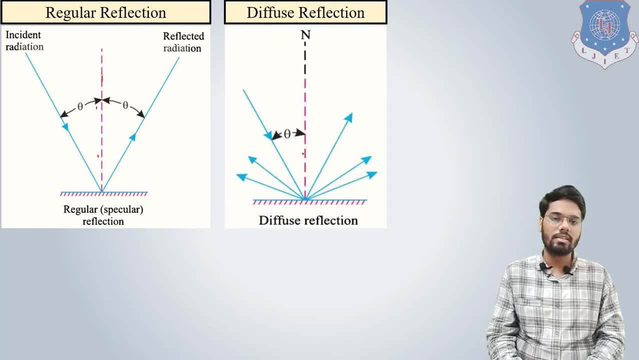 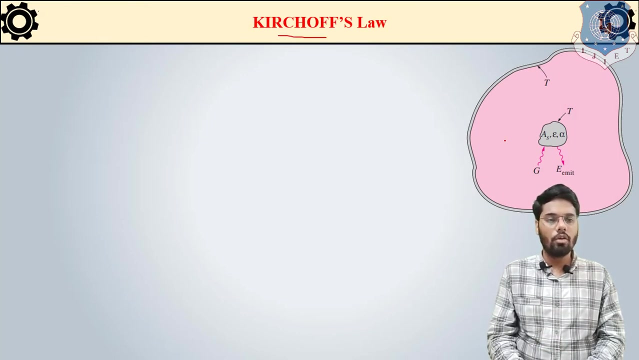 and second one is a diffuse reflection. here from figure you can understand what is diffuse reflection. the the angle which is made by incident radiation and the angle which is made by a reflected reflector, electromagnetic wave is differed, so that is known as the diffused reflection in all direction. now one more important law is a kirchhoff law. here from the figure you can see: 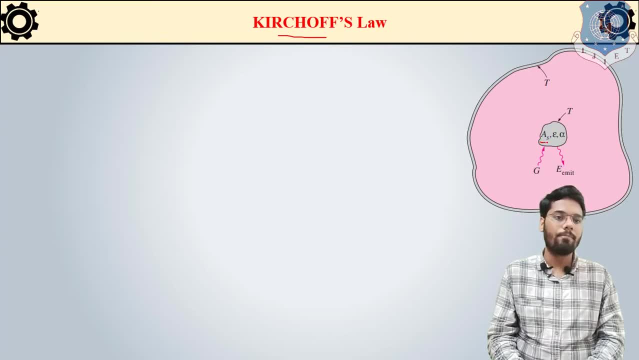 that there is a one small body whose surface area is air, and so the surface area is a surface area whose emissivity is epsilon, whose absorptivity is alpha, is it? it is enclosed by one another body whose temperature is capital T, which is isolated from the surrounding. now the radiation incident. 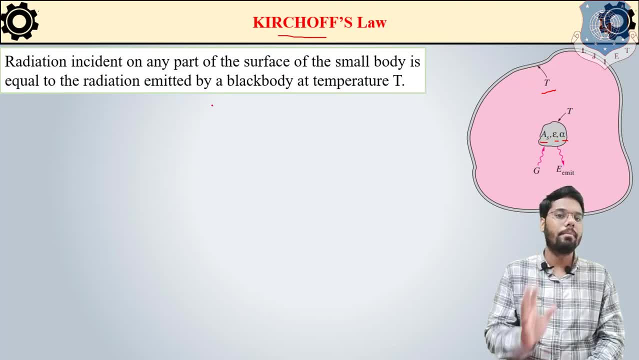 on any part of the surface of small body is equal to the radiation emitted by a black body at temperature T. this black body, whose temperature is T, whatever amount of electromagnetic wave is emitted from this black body, will going to incident on this small body whose surface area. 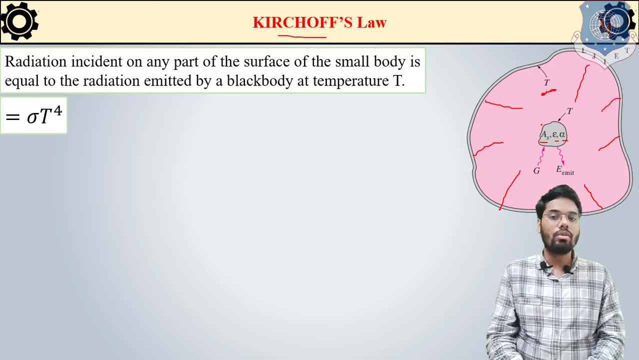 is air and that amount is going to be sigma into T raise to 4. from this different Boltzmann law we know that the emissive power of black body, which can be calculated by sigma into T raise to 4, this all radiation will absorb by this small body per unit area, per unit of its surface area. so the 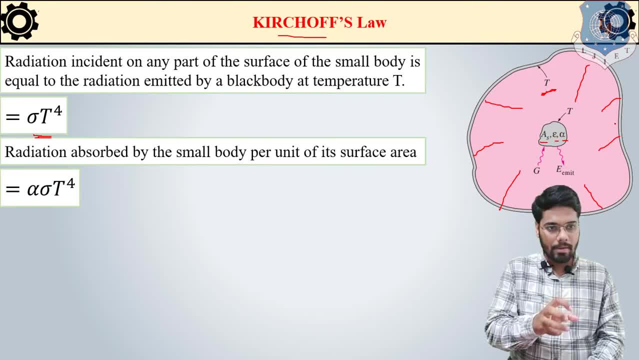 amount of electromagnetic wave which is coming from the black body is equal to the amount of electromagnetic wave which is coming from this black body to this small surface area, is to this body. the amount of that electromagnetic wave which is going to be absorbed by this body will be alpha into sigma, into T, raise to 4. alpha is ability of this small body to 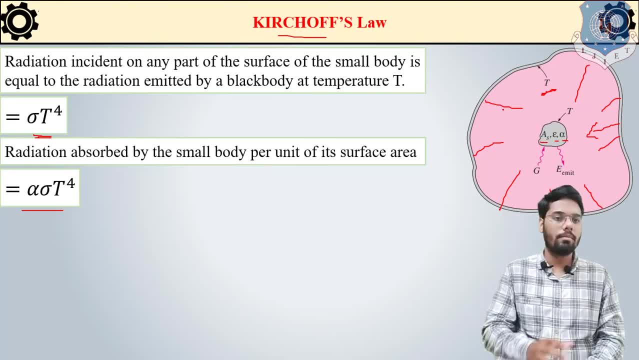 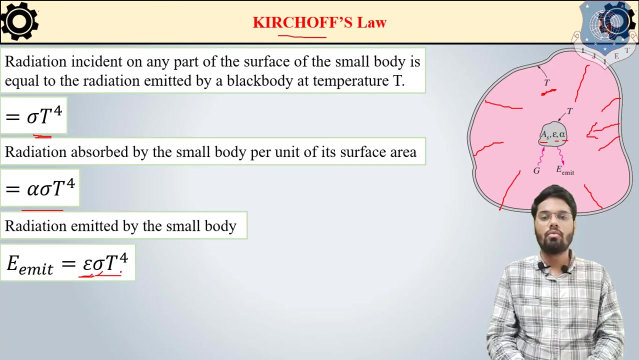 absorb the electromagnetic wave which is coming from the surrounding, which is coming from this black body. now there are some radiation which is emitted by this small body, because it is 0, so amount of electromagnetic wave, or we can say that amount of radiation which is emitted by this a small body is its emissivity into sigma, into T. raise to 4 for black body, is sigma into T. 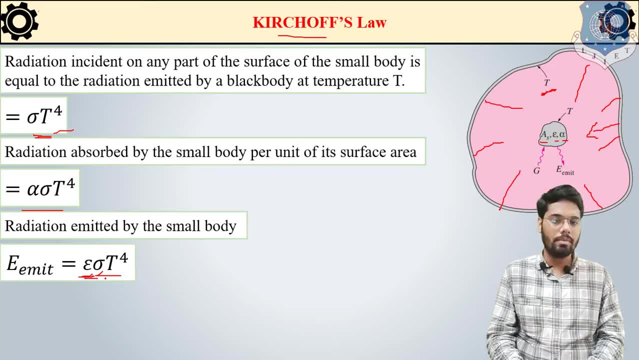 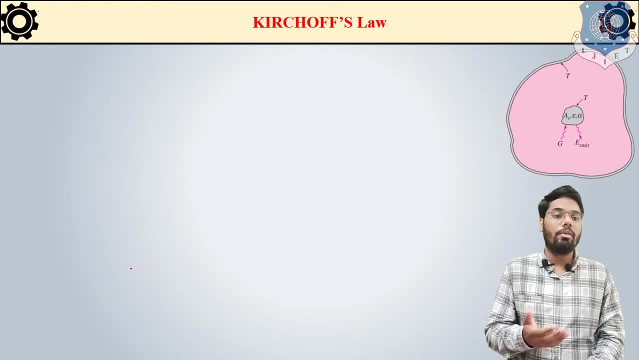 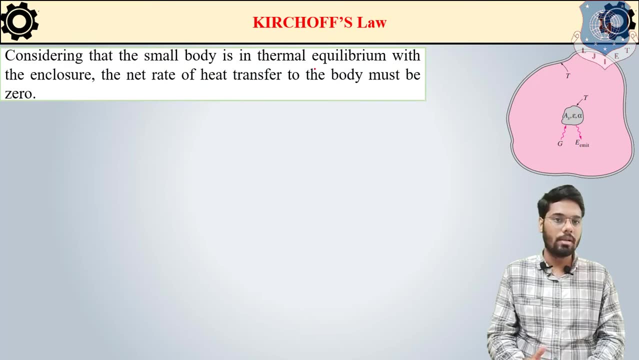 raise to 4. for real bodies it is epsilon emissivity into sigma, into T raise to 4. so now we know that whatever electromagnetic wave emitted by this body will be absorbed by the, this black body. So, considering that small body is the thermal equilibrium with the enclosure, we know that. 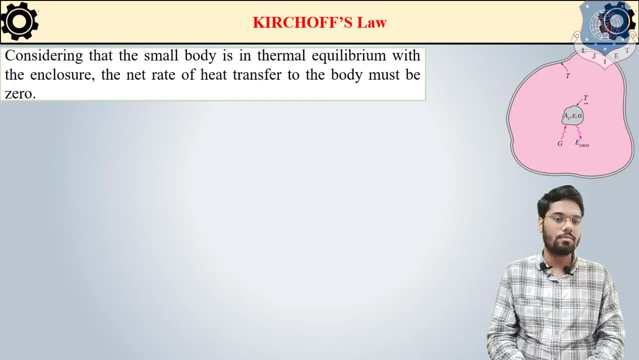 both temperature of both this body and the black body is T. So this: both bodies are in a thermal equilibrium. So for thermal equilibrium the net heat transfer between these two bodies should be zero. So, whatever the radiation emitted by the body must be equal to radiation absorbed by the 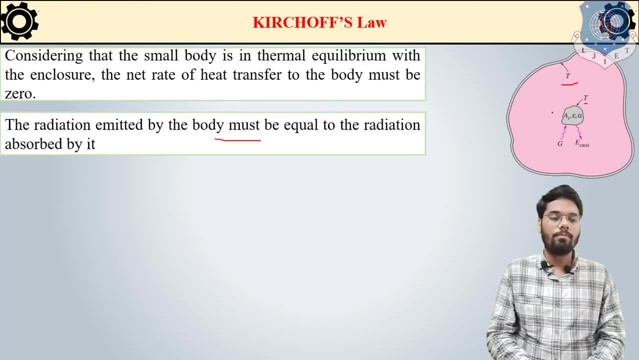 body, Whatever, I repeat once again, for thermal equilibrium, because this black body is at temperature T, this real, this is our body, which is at also temperature T. So this black body and this real body, both are at temperature T, which is in thermal equilibrium. 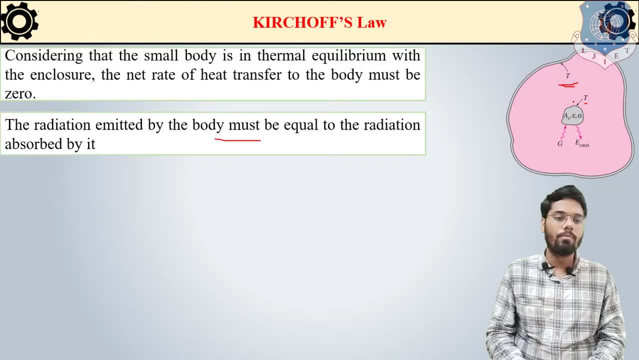 So the net heat transfer between these two should be zero. So whatever amount of electromagnetic wave, or we can say that whatever amount of radiation absorbed by this body because of radiation of this black body equal to radiation emitted by this body. So we can write that. 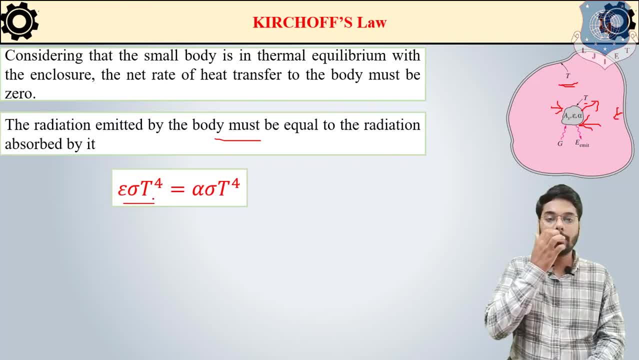 So we can write down epsilon into sigma, into T, raise to four, which represent the amount of radiation emitted by this small body, is equal to alpha. into sigma, into T raise to four, which is absorbed, or radiation absorbed by this body from the black body. 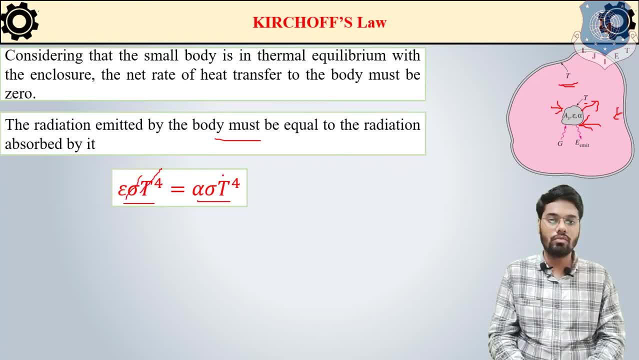 So from this equation, sigma into T raise to four, sigma into T, raise to four would be cancelled out. So remaining would be absorptivity. emissivity is equal to absorptivity. So whenever two bodies Which are in thermal equilibrium 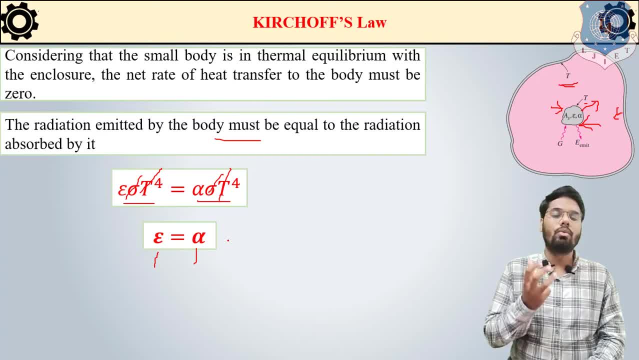 At that time, emissivity of body is equal to absorptivity. absorptivity, See it simply- means the body who is in thermal equilibrium with the surrounding. at that time, the amount of electromagnetic wave which is emitted by the body is the same as the amount 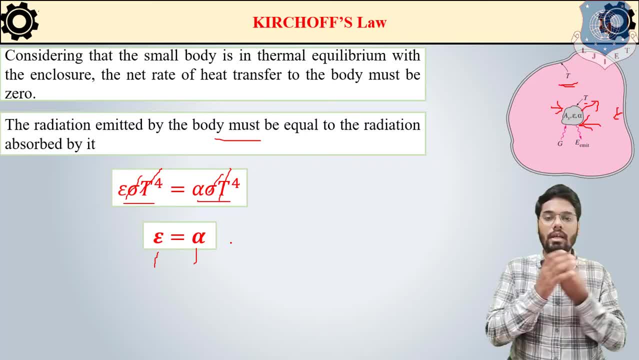 of electromagnetic wave which is, because of which is incident on the body, or which we can say that which is absorbed by the body, so that the temperature of that body with surrounding will remain in a thermal equilibrium. and this law is known as the kirchoff's law, which 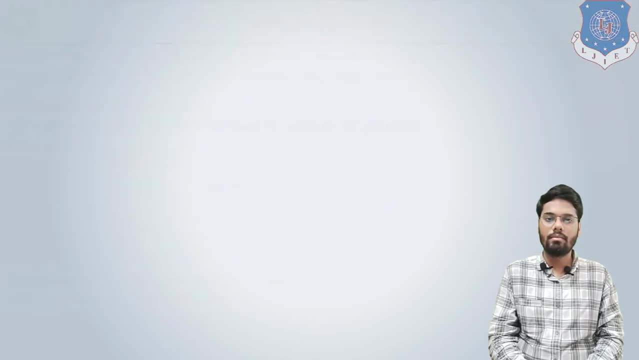 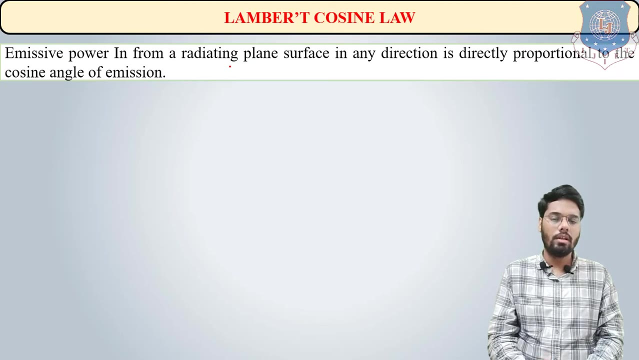 is developed in 1860.. now one another law is lambert cosine law. it is a simple law. emissive power in form of in from radiating plane surface in any direction is directly proportional to the cosine angle of emission. generally, a body whose temperature is about 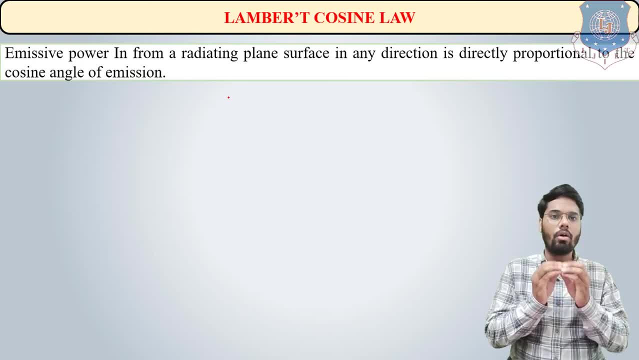 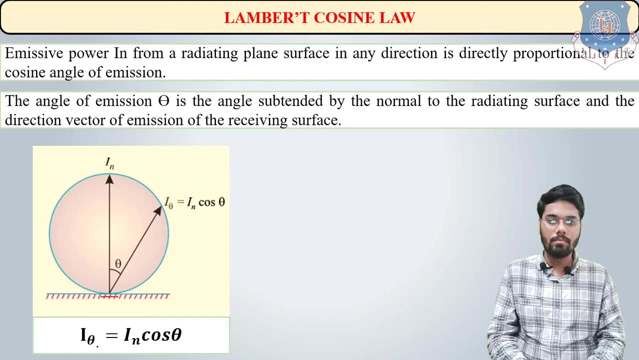 absolute zero temperature emits electromagnetic wave in all the directions, but the intensity of electromagnetic wave in a normal direction is highest as compared to other direction. so if from this figure we can see that, if this, if we consider electromagnetic wave emission from this point, the intensity is in normal direction, is the highest intensity, which is denoted by the in. 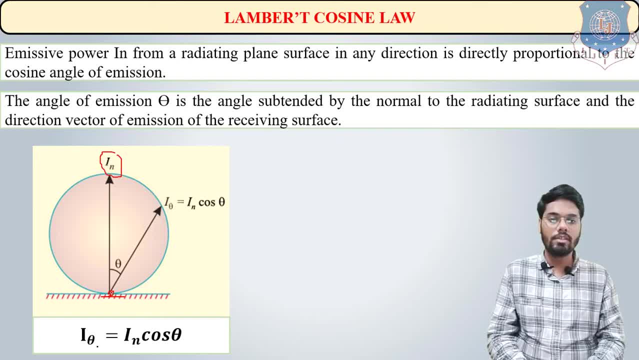 now, if you want to find out the intensity of radiation from this point, at particular this, this point it means from- it is a from angle, normal angle is theta. so from this point, at theta angle, the intensity would be in cos theta, which is denoted by i theta, the intensity of radiation from this point for the theta angle. 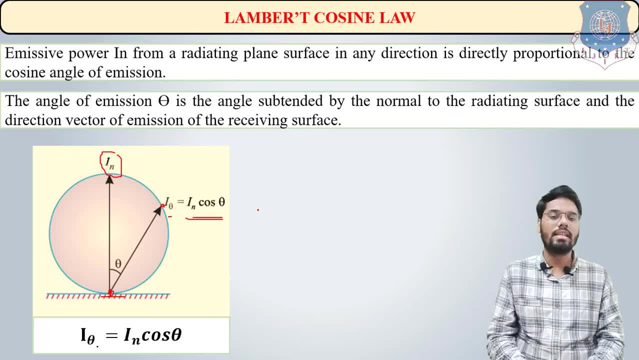 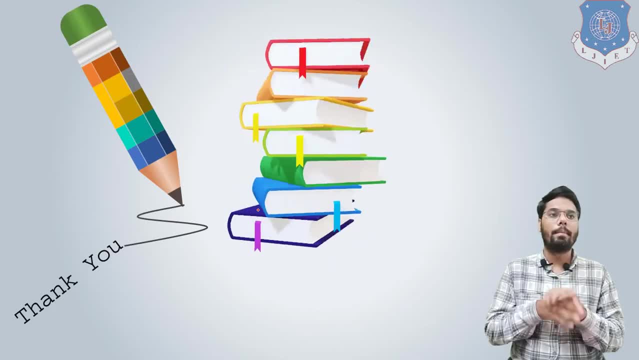 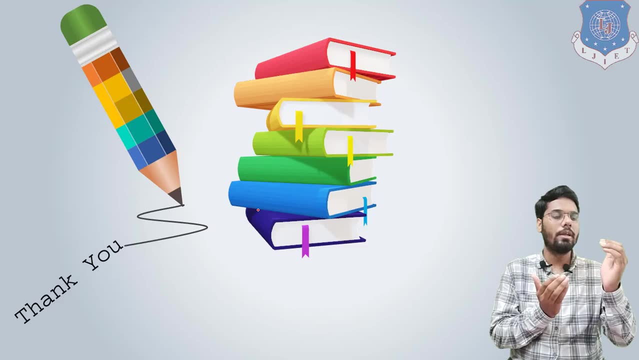 would be written as i n cos theta. this law is known as the lambert cosine law. so that's it for today's lecture, today's session. in this session we have learned about the black body radiation. why we have studied black body? because for the reference point we need one standard body to which another radiative. 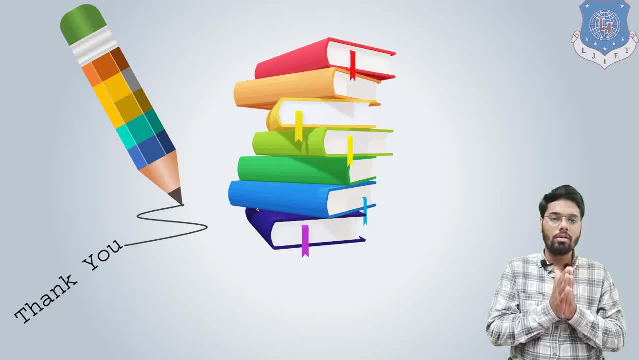 properties of real surfaces can be compared because and we also learn that all the bodies whose temperature is about absolute zero emit electromagnetic wave and that electromagnetic wave contains energy. now, amount of electromagnetic wave, or the wavelength of electromagnetic wave, it depends on the different emission properties, like surface material, of the surface surface.